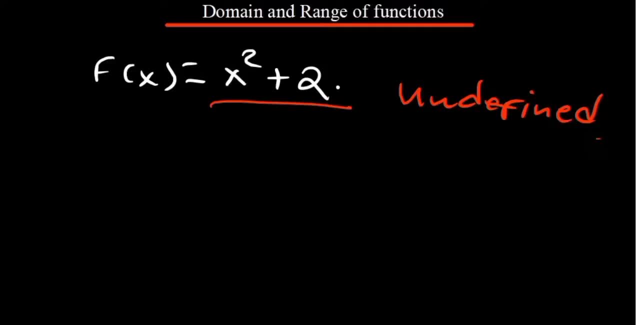 Okay, so in this case we don't have any limitations. Any value of x, whether negative or positive, it can still give us A result. So therefore we can say: our domain in this case can be a set of all real numbers. 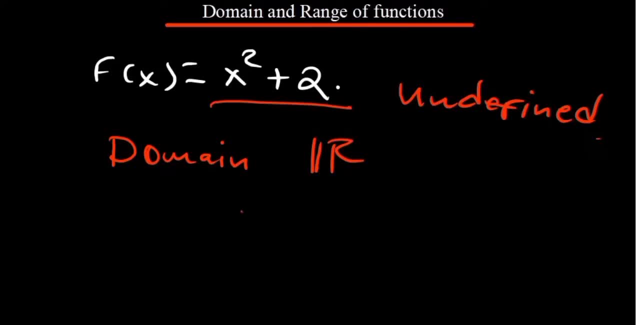 Okay, which you can present as From negative infinity. This is less than x, Then x is less than So. this is in terms of set interval notation. The other way you can say is you can use this: You say x is a member of. 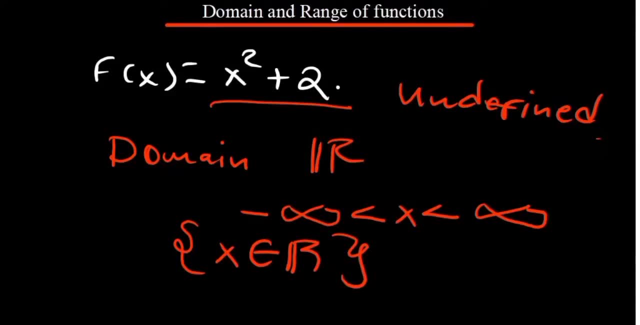 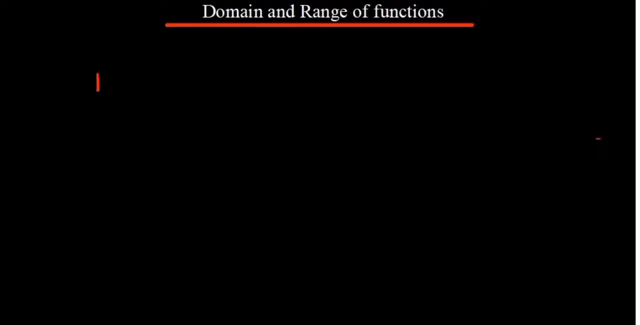 Real numbers. Okay, so what is the domain in this case? Alright, Now Let's say you've been told that Determine The domain, the range of that function. So we are therefore x being equal to x squared plus 2.. 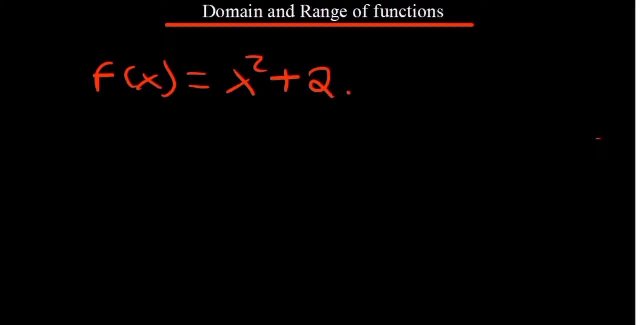 So how do we now determine the range? So the range, you just have to first of all come up with an inverse function. So remember why It's equal to x squared plus 2.. So our goal in this case is to make now x a subject of this. 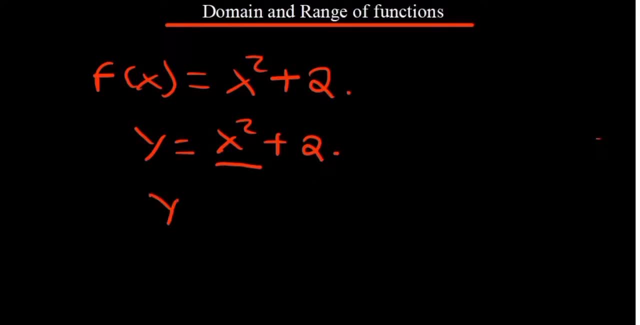 Of the formula. So what you're going to have is y minus 2. Being equivalent to x squared. So if you make x a subject, it's going to be The root of y minus 2.. Okay, so this is now. 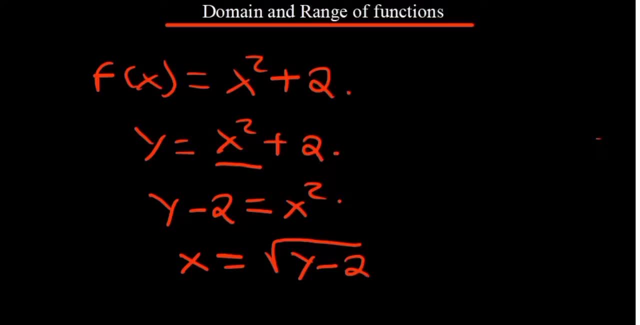 The inverse function Of that Of course we need. In cases where they've asked you to determine The inverse function, You're supposed to present it in this form, So where there is a y, you put x now, But that is not our interest in this video. 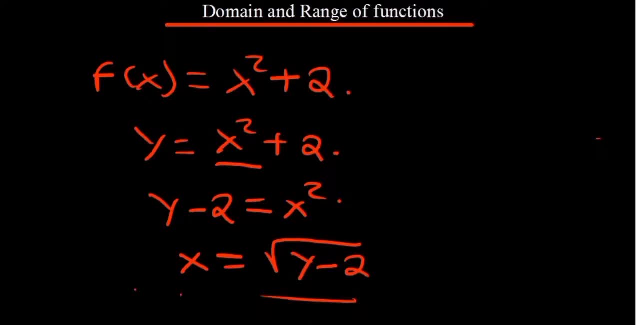 So let's try to, Let's try now to determine the range. So, the range, We are just going to look at it in the point of view Just as we determine the domain, So, except what we have as our function is, 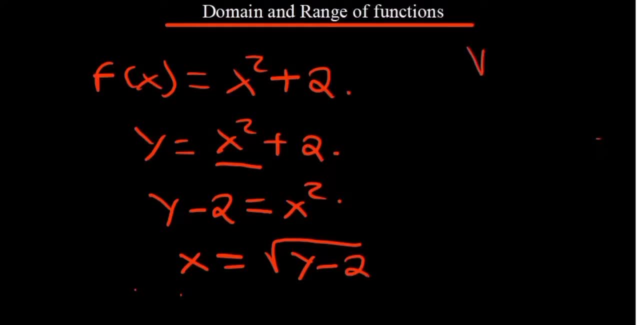 The root of Y minus 2.. So are there any limitations? Is there anybody that can make this function to be undefined In terms of the real numbers? Okay, so Whenever you have this root of a negative number, It's undefined under real numbers. 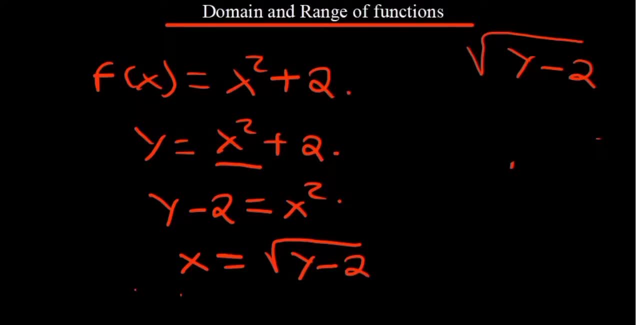 So when you're talking about functions, We're not interested in complex numbers, So we can say that All the values That are Under a square root Should either be equal to 0. Or greater than 0. So we should say: y minus 2 should either be greater than or equal to 0.. 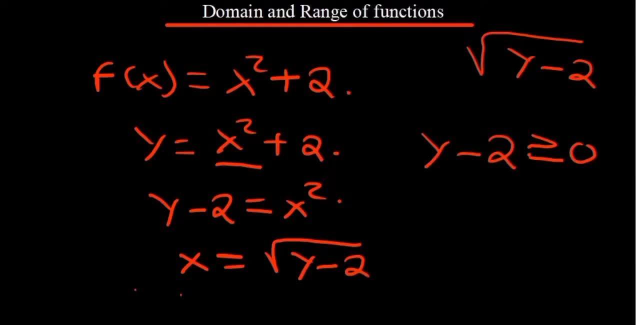 That's what we want. So we are going to see that Y Is actually going to be Greater than, or equal to, 2.. Alright, So these are the values That we should expect to be under a square root. 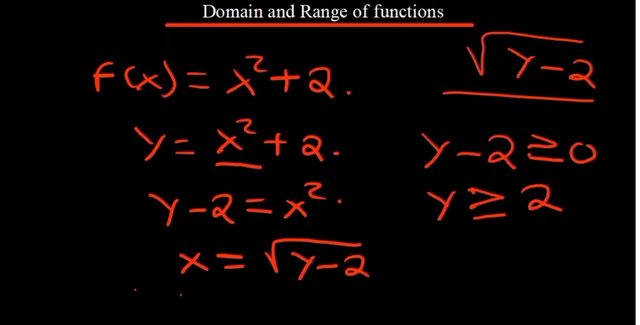 For it to be undefined. So how do you present it now? as the range. So you can therefore say: Your range in this case of that function is going to be So here is where you can put the function itself. So we expect that all the values that you are going to have inside that function 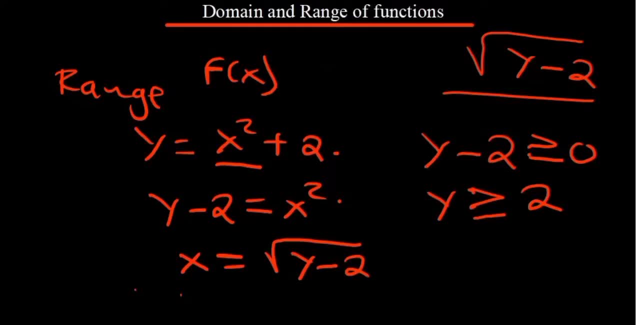 Are supposed to be Greater than Or equal to 2.. So the minimum value that you have is 2. And all the other results are supposed to be greater than 2.. And that makes sense if you look at this function. 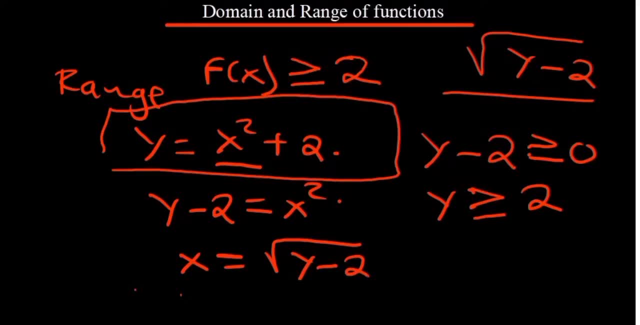 So you expect that, whether you put a negative or a positive number, They are all going to be To give you a positive number at that point, And so the minimum that you can have is when x is equal to 0. And that is your 2.. 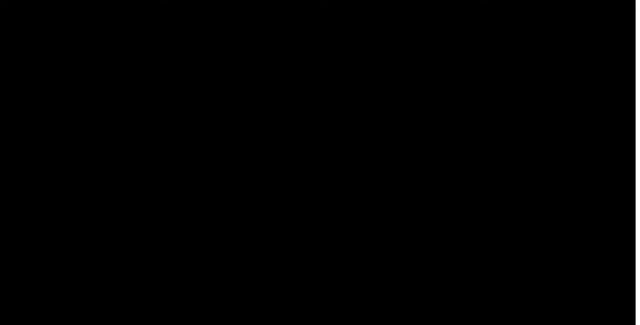 So that makes sense. Now let's say You have The function Of x being equal to x plus 1. Divided by 2 minus x. I have asked you to determine the domain And the range. So to start with, 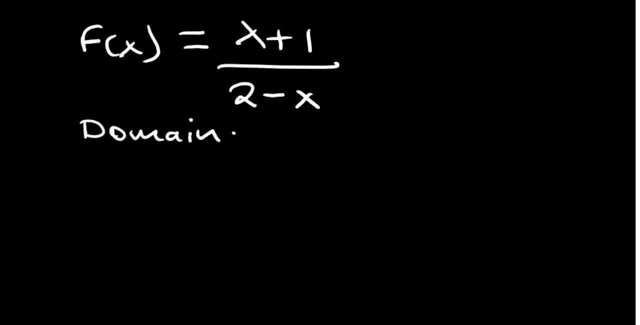 How do you determine the domain? So think of it in this way. Think of it from a negative point of view. Is there anything that can make a fraction to be undefined? So we all know that a fraction is undefined when you are dividing by a 0.. 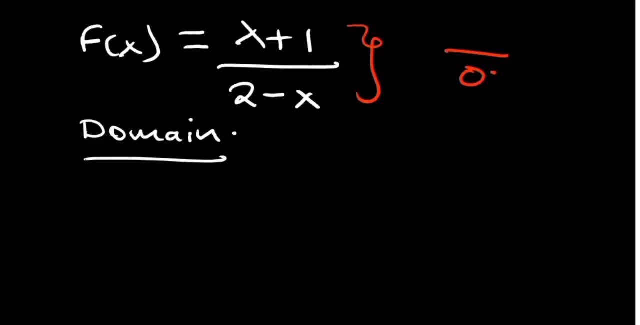 So we should come up with a set of x values that should not give us a 0.. On the bottom, On the denominator part: So 2 minus x Therefore Should Not be equal to what Should not be equal to 0.. 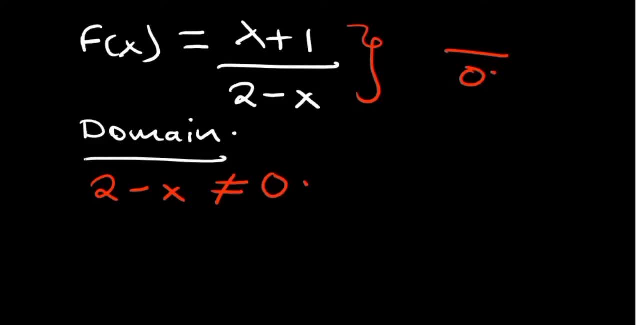 Should not be equal to 0.. Should not be equal to 0. So if you make x to be a subject, You have negative x Being Not being equal to Negative 2. So you divide by The negative on both ends. 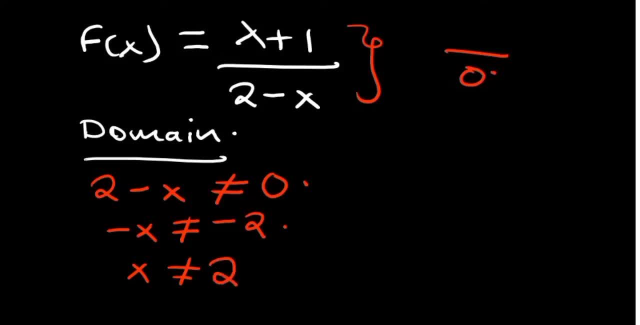 X is actually Not supposed to be equal to 2.. So all the other values can work except 2. Because if you put 2 where there is x, It is going to be a 0. Which is going to make it undefined. 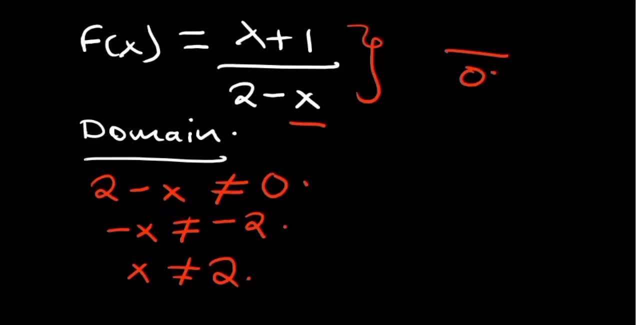 So we can therefore say That x is a member of real numbers, But x should not be equal to what Should not be equal to 2.. So that's our domain for this function. Okay, How about the range? How do we get to determine the range? 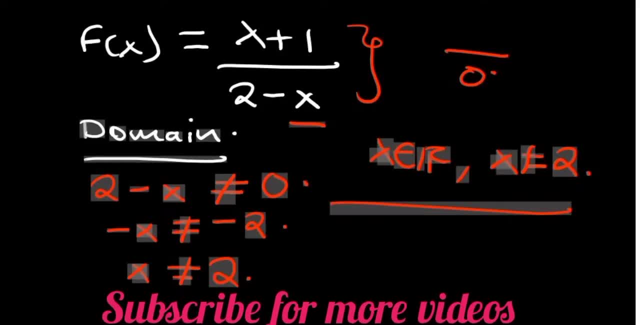 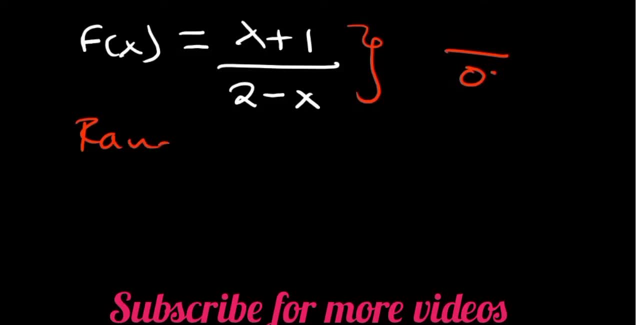 So the range in this case Is supposed to be dependent, Dependent on the inverse function. So Let's try to make x a subject, So let that part for the function be y, So y is equal to x plus 1.. 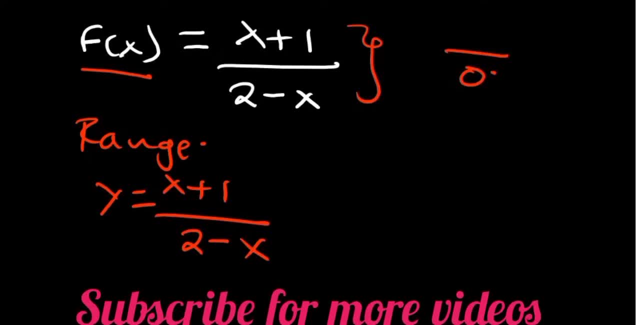 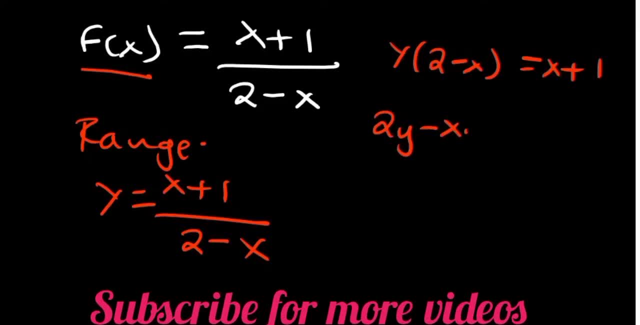 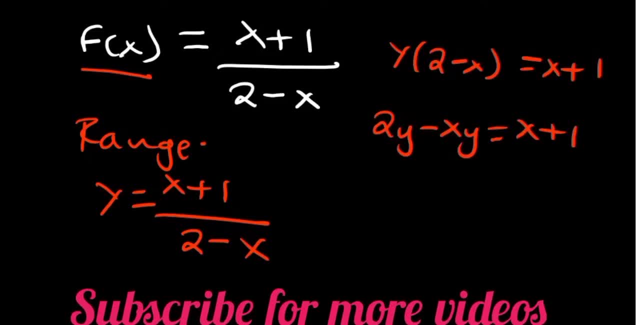 So remember our goal is to make x a subject, So this can go the other side there And the one can go the other side. So we have 2y Minus 1.. Is equal to x plus x y. 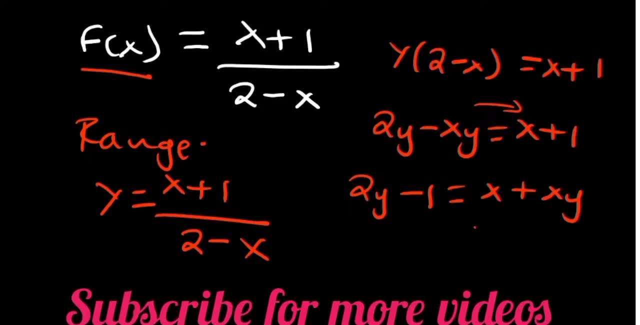 So, making x a subject, We can factorize it And remain with 1 plus y. On this side we maintain what we have: x plus 1.. x plus 1.. So from there we are going to see that we are going to have. 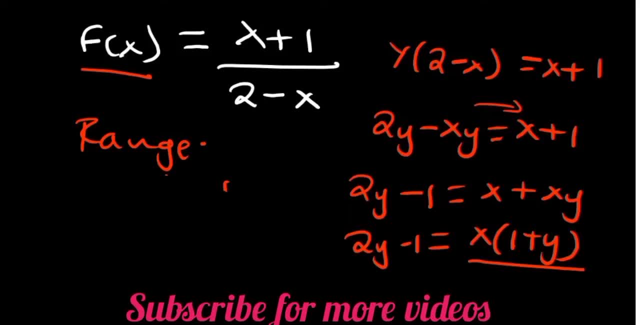 So if you divide on both sides by 1 plus y, Because our goal is to make x a subject, So 1 plus y. So your x is therefore equivalent to 2y minus 1 over 1 plus y. 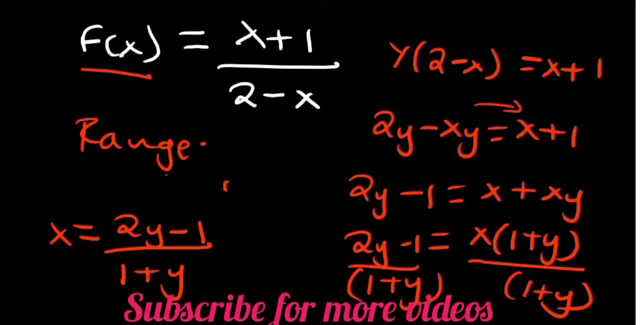 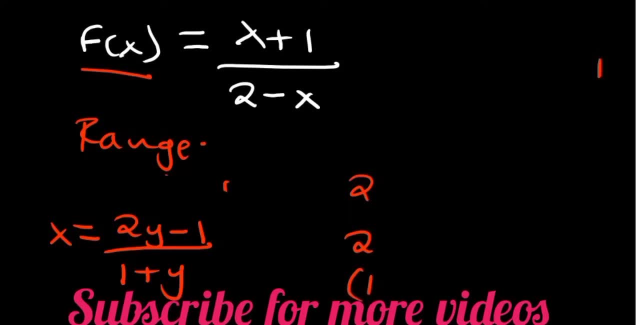 So you've come up with an inverse function in terms of y. So you've come up with an inverse function in terms of y. So let's try to determine now the range. So, just like we determined the domain, Even the range, you are supposed to do the same. 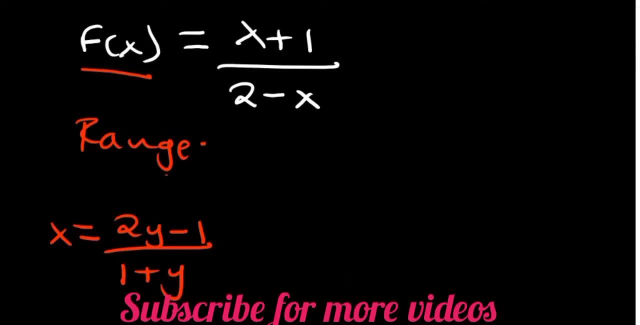 So, when you have a fraction, What your goal is? to make sure that you don't have 0 as a denominator, Because it is going to make a function to be undefined. So 1 plus y, Which is the denominator, Should not be equal to 0.. 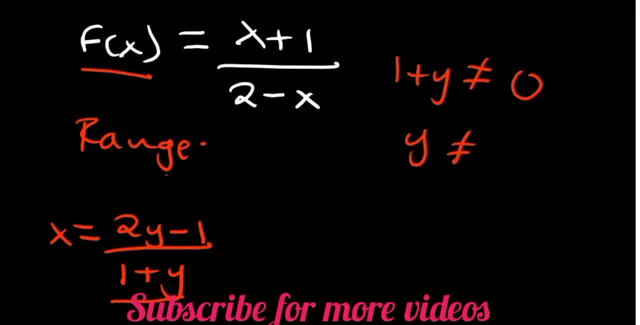 So y is therefore not supposed to be equal to negative one. okay, so what can we say? we can therefore say that the range f of X- the values that we should expect- are, of course, member of all the real numbers, but we expect that the function is never equal to what it's never equal to. 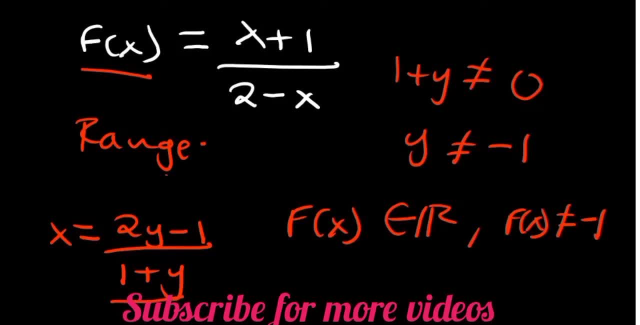 negative one. so there's no value that is going to give us a negative one in this function and this is therefore your range of value. so what is the range? so the range is giving you a set of Y values that you should expect in a function that you are given okay. so the possible results are all real numbers. 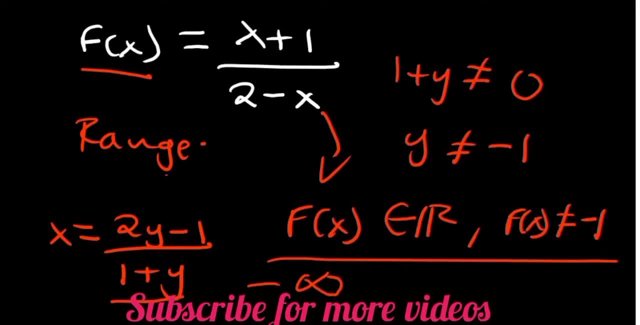 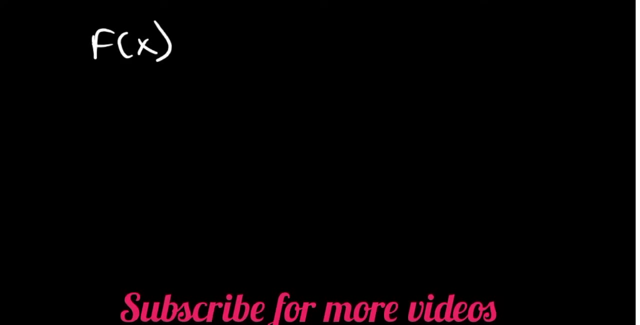 between negative infinity all the way up to two positive infinity, except the function is supposed to skip negative one. that's what it means. now let's say you've been given a function- one plus x, squared plus one, so you can pause the video and try this one out, all right. so if you look at it as 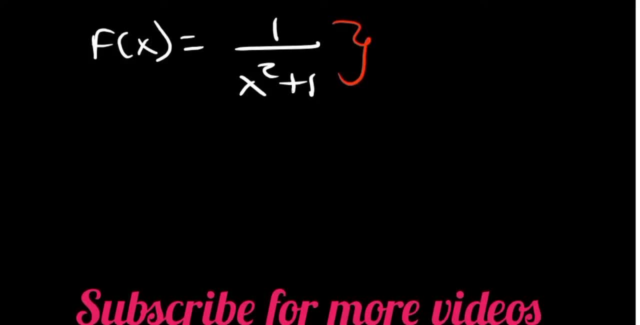 well, it's also a function, so we expect that we shouldn't average nominate about. is that equal to zero? so therefore, our domain, we expect that x squared plus 1 should not be equal to 0. so x squared should not be equal to negative one. so 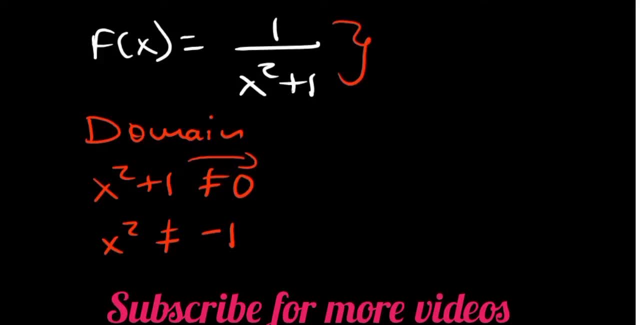 So that has gone the other side. Okay. So what else can we say? Our goal is to make a, So our goal is to make a x. the subject, So x should not be equal to root of negative 1.. 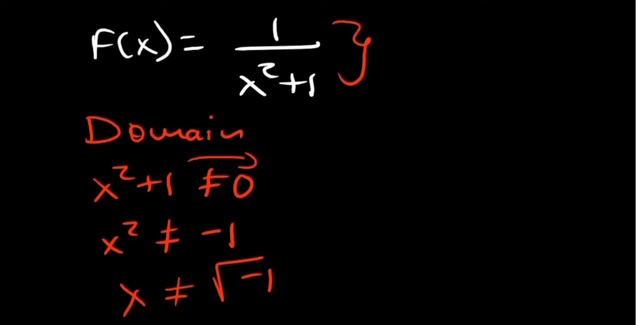 So what does that mean? So that means that there is no value that you can put there. where is x squared Apart from the root of negative 1.. So- and this is not part of real numbers, It's a complex number. 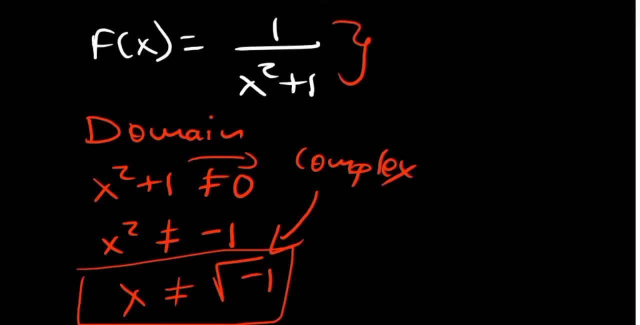 So it being a complex number, So there is no real number that can make that function to be undefined on the denominator part. So we can just therefore say that the domain is a set of all real numbers, From negative infinity to positive infinity. 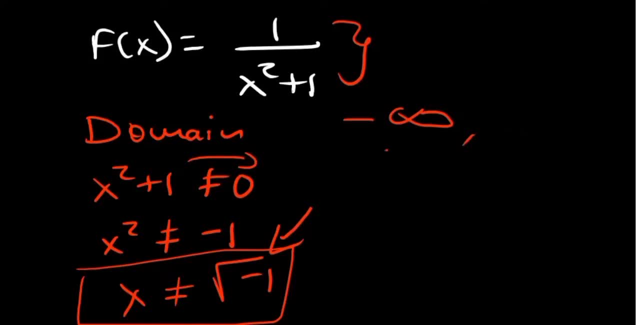 Of course we use caved brackets. So if you don't know how to present sets using set in double notation, Check out for a video on that. Okay, So the other way we can say our x values are actually a member of all real numbers. 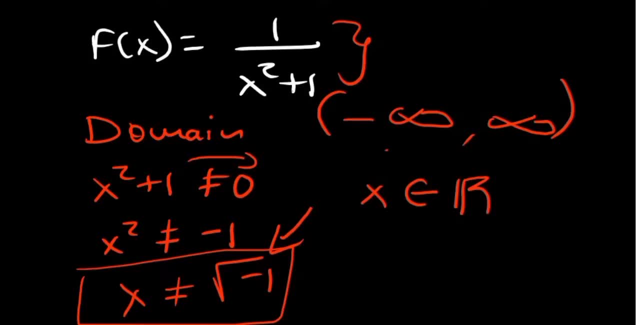 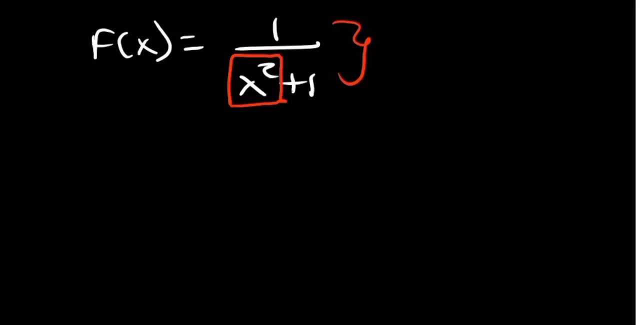 There is no exception. Okay, So that is our domain in this case. So there is no value that you can put. where is x squared to give you a 0. Because it has given us a complex number. How, then, can you find the range of such a function? 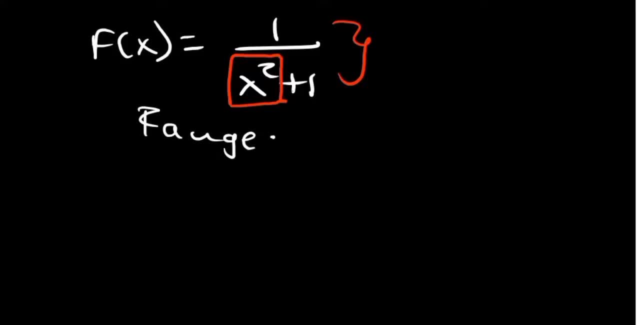 So, like as usual, The range is supposed to First of all make x a subject of a formula. So where there is a function there, we put y over x, squared plus 1. So you have y, x squared plus 1.. 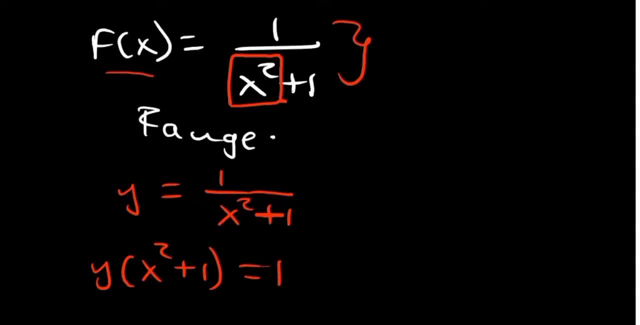 Of course that multiplied there. So if you make x to be a subject in such a case, So you have to distribute y, So it's going to be y x squared. Let me write that on top: So y x squared. 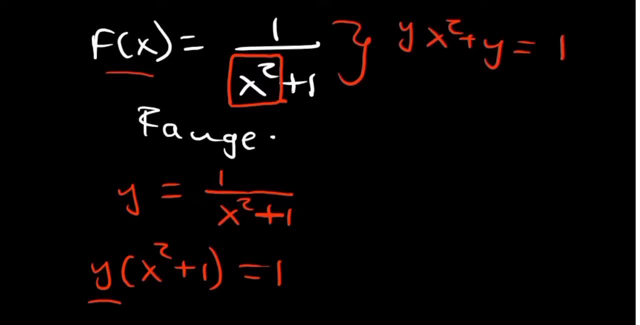 Plus y Equal to 1.. So our goal is to make x a subject. So you remain with that. on the left You have 1 minus y. So you divide by y And your x is going to be the root of 1 minus y over y. 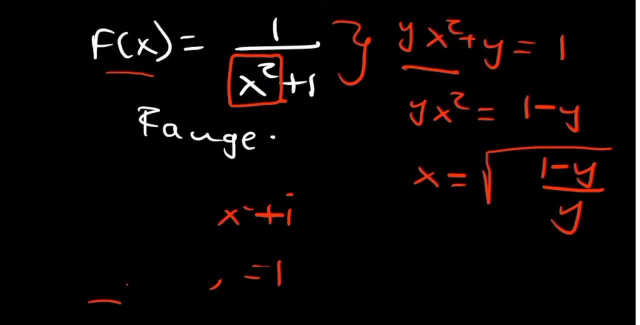 So we've come up with the inverse function in terms of y. So we need to look at the values that can make a function to be undefined. So we have a combination of a fraction As well as a square root. So in a square root for real numbers, we shouldn't expect to have a negative number there. 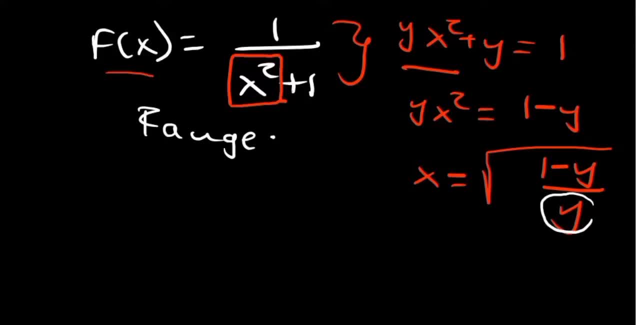 And for a fraction, we don't expect y to be equal to 0.. So these are some of the restrictions that we have. y should not be equal to 0. Then 1 minus y has a fraction Should be greater than or equal to 0.. 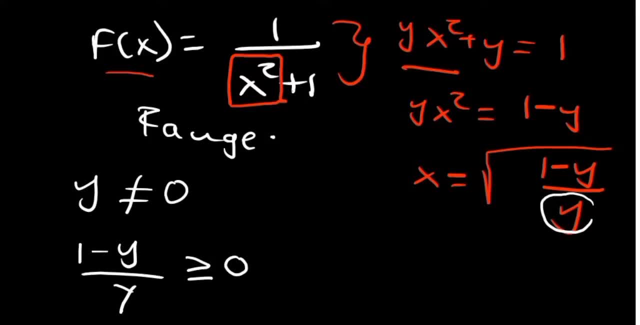 Because we don't want negative numbers there. So we need to find the values of y that we should expect after plugging in the values of x in that function. So even before solving, if you look at that function, it's 1 over x squared plus 1.. 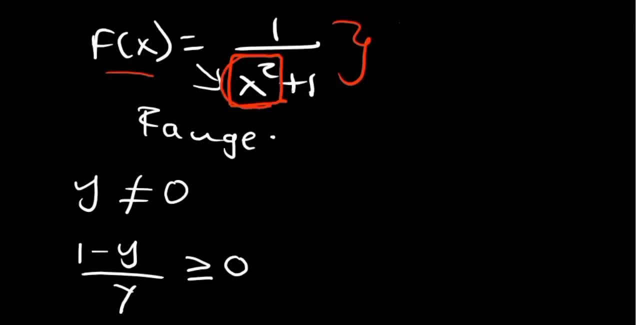 So all the values that we are going to put in under x, squared, whether positive or negative, they are still going to give us positive numbers. So, first of all, all we should expect are positive numbers, But then the maximum number that you can have should be 0.. 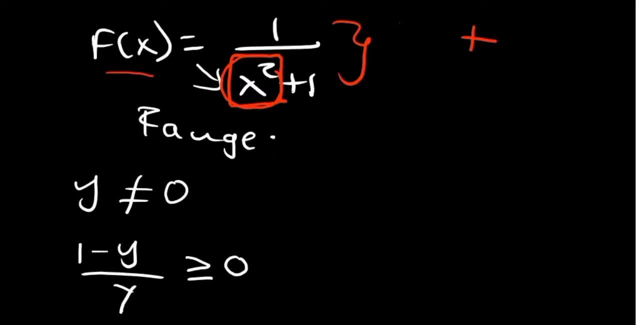 Should be a 1, sorry, Should be a 1.. When x is equal to 0,, you have 1 over 1,, which is just going to be a 1. As the biggest number that you are going to have. 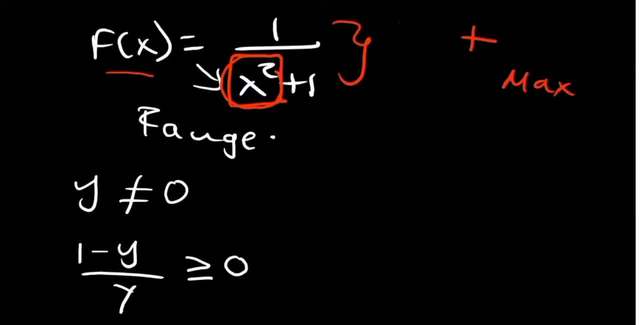 So you have a maximum number to be 1.. Again, we don't expect to have negative numbers, So it's just Less than 1.. So x should be less than 1.. Then it's also equal to 1.. 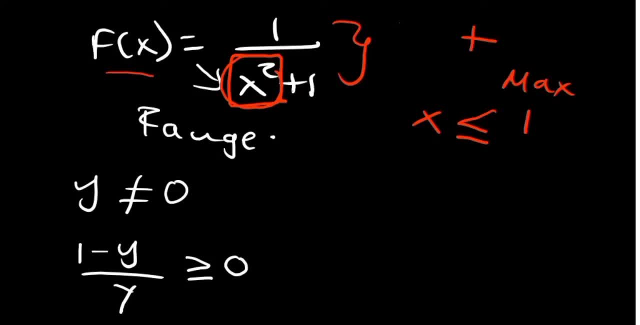 But then what is the minimum value that we expect? So do we expect to have 0 in this case. So there is no possibility of having a 0. Unless if we add x on top. But in this case there is no possibility of having the function being equal to 0. 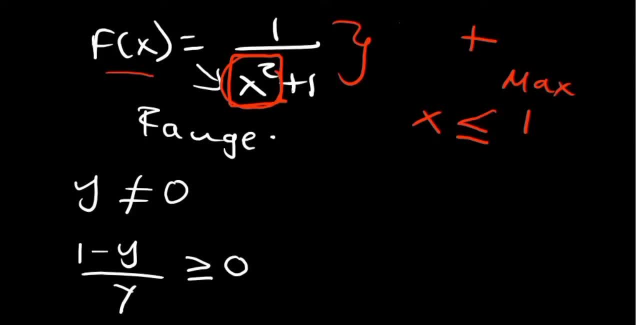 But numbers can't go beyond 0.. 0 is less than x, but x is greater than, is less than or equal to 1.. So this is your range that you should expect. So now let's try to determine that by solving by calculations. 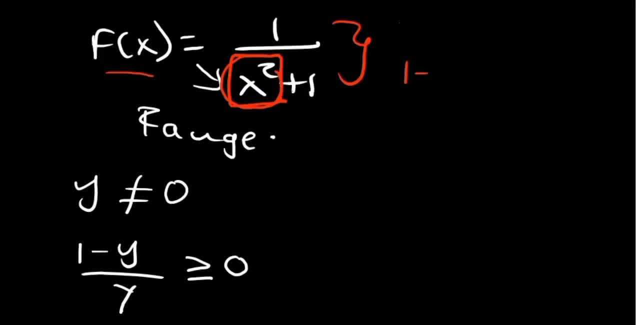 Okay, So we have 1 minus y. over y, It should be greater than or equal to 0.. So what we are trying to solve here is An inequality. So if you've not looked at inequalities already, do well to check out our video on that and you'll be able to understand. 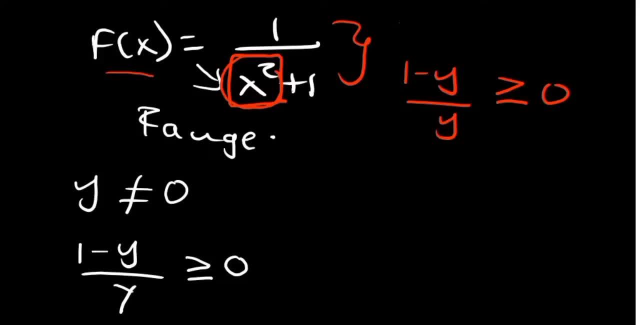 Okay, So we solve inequalities equated to 0 by getting the numerator. So 1 minus y should be equal to 0. So that we determine now the distinct points. So, making y, the subject y is going to be equal to 1.. 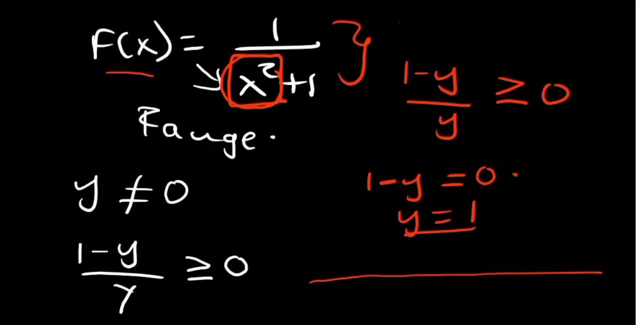 Okay, So come up with a number line So we have 1.. Okay, Another point. What other points can we use? We can use 0 in this case, because we know that there's no possibility of having a 0.. 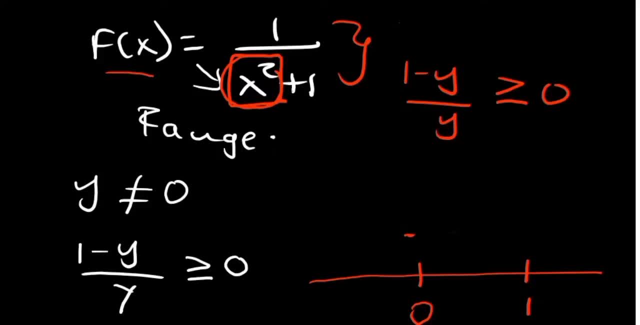 So we can use that. So the only possibilities of us are: So it's either the numbers are between 0 and 1. That can give us a value that is greater than 0. Or less than 0 or greater. 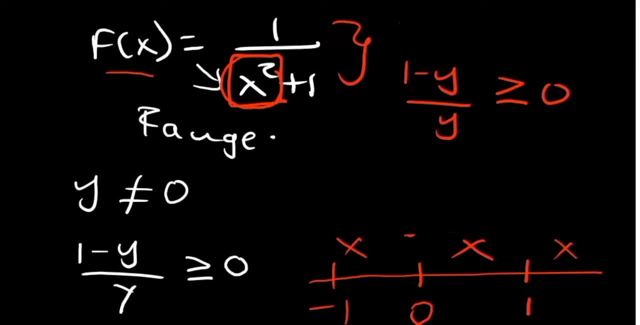 So I'll start with less than 0.. Negative 1.. So if you plug in negative 1 in this function, what value are you going to have? 1.. So we plug in negative 1 over negative 1.. 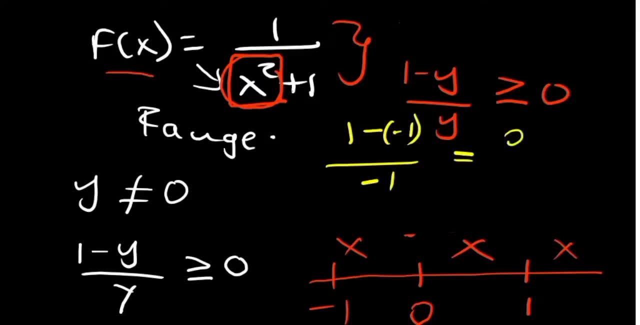 So you have 2 over negative 1, which is negative 2. So that value is less than 0. So this part is disqualified. Alright, Let's get a number Between 0 and 1. Let's say maybe 1 over 2.. 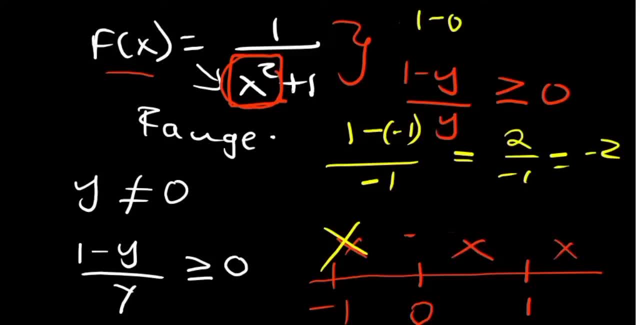 0.5.. So you have 1 minus 0.5 over 0.5.. So 1 minus 0.5 is 0.5 over 0.5, which is giving us a 1 there. 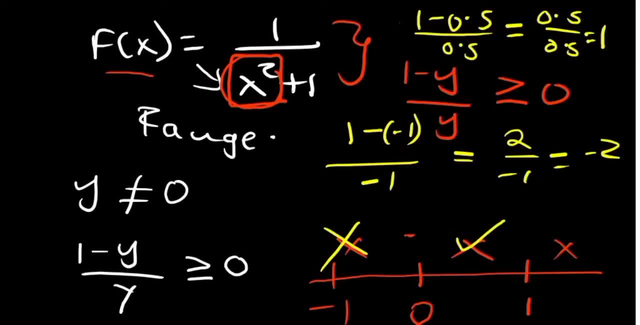 Okay, So this part is giving us a positive number. How about greater than 1?? Sorry, So, if you try, maybe 2.. 1 minus 2 is negative. 1 over 2 is a negative number, So we don't want that. 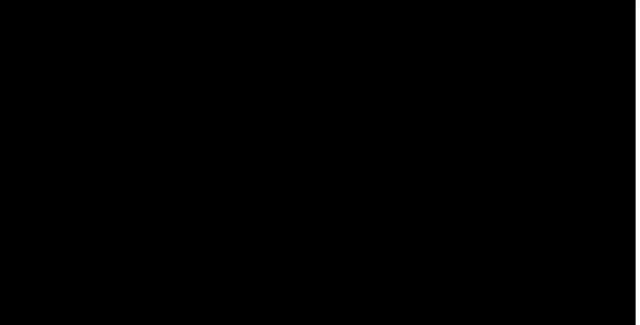 So we can therefore make a conclusion to say the only numbers that we need, they should be greater than, So our function result should be greater than 0 and should be less than or equal to 1.. But 0 is not included. 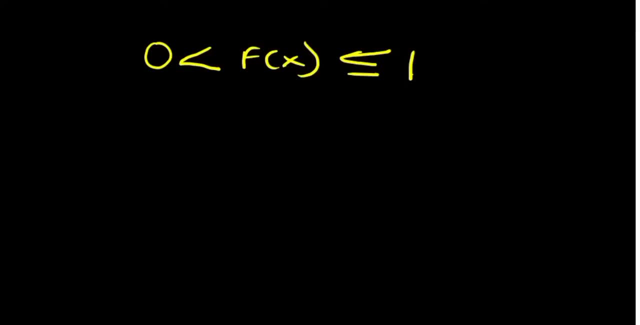 That's why we've not put this there. Now let's say you have f of x being equal to the square root of 1 minus x squared. So we ask you to determine the domain of such a fraction. How do you determine the domain? 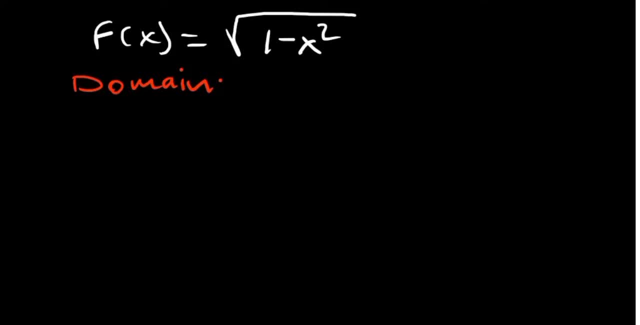 So we're saying that whenever you're given a square root, we're supposed to make sure that whatever is below there is supposed to be greater than or equal to 0. So we don't want to have a negative. So we don't want to have a negative. 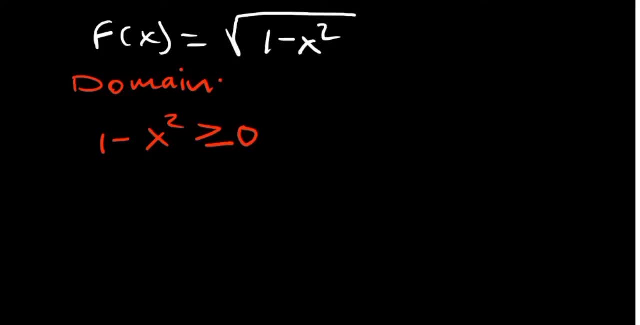 So we don't want to have a negative, So all the numbers that we want are supposed to be greater than or equal to 0 itself. Okay, So how do we solve inequalities? So, if you're not so confident, check a link for the video, for a video on inequalities. 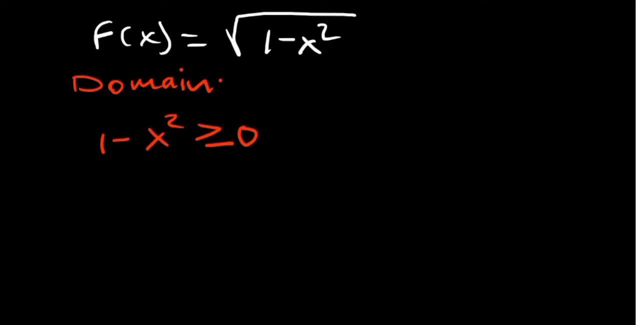 So whenever you have such an expression there, it's very important that you come up with distinct points. Okay, So rate this part be equivalent to 0. So 1 minus x, squared being equal to 0. That is possible. 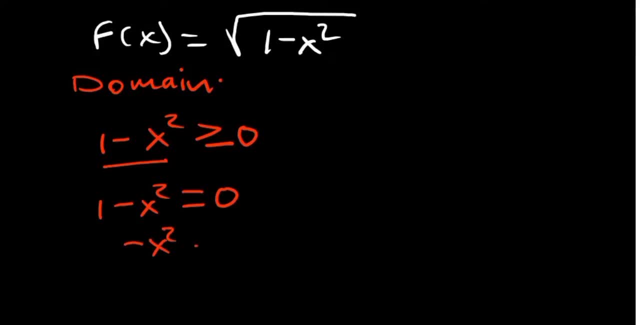 So negative x squared is going to be equal to negative 1. So you divide both sides by negative 1. x squared is equal to 1. So our value of x is going to be plus or minus. the root of what? 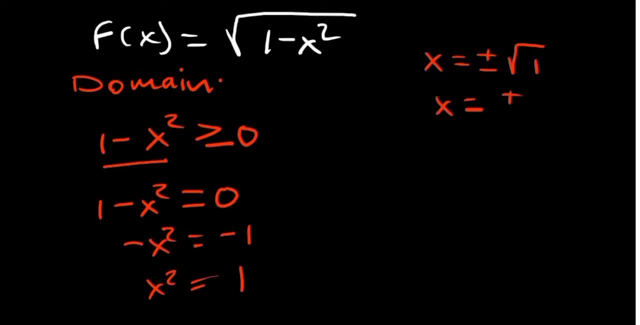 1. So what you have is positive or minus 1. So you come up with a number line. You have a negative 1. You have a 1 there. So it's either They are less than in between or greater. 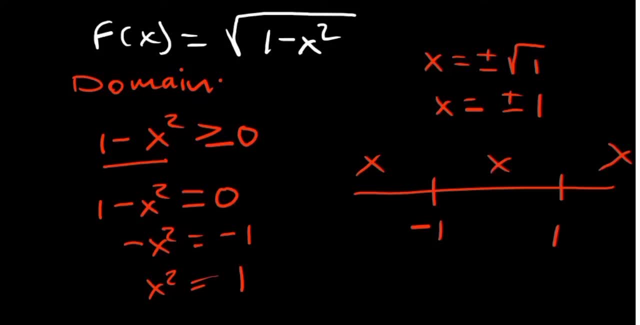 So those are the possibilities that we should expect. So let's try out and see which values can give us the numbers that are greater than 0.. Okay, So I'll start with in between, I'll start with 0.. 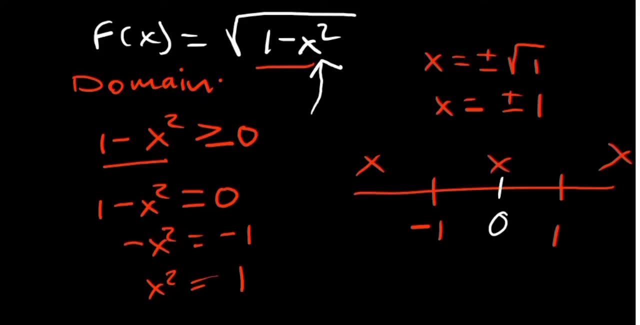 So what happens if I plug in a 0 here? What should I expect? So if I plug in a 0 here, Suppose we are going to have 1 minus 0. And the root of that is going to be a 1..